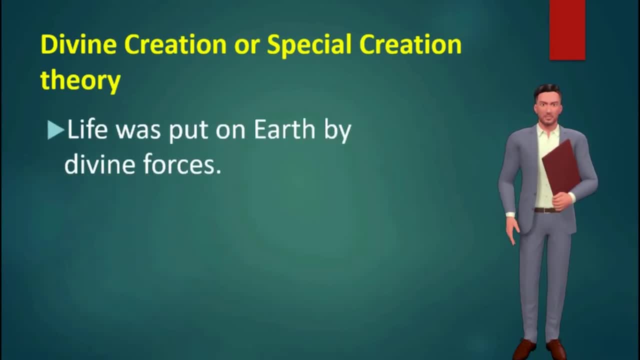 life was put on Earth by divine forces. Creation theories are common to many of the world's religions and cultures. In this theory, it says that God created everything, including life on Earth. The fourth theory of the origin of life is the origin from nonliving matter or spontaneous. 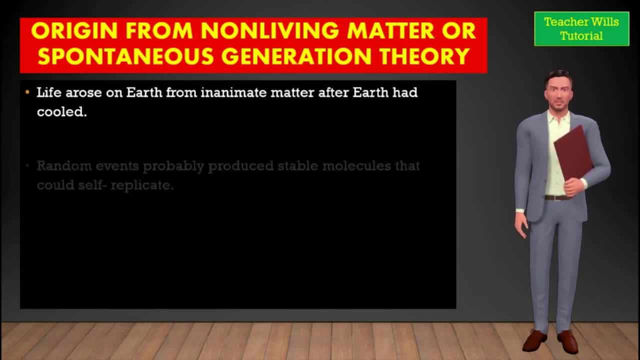 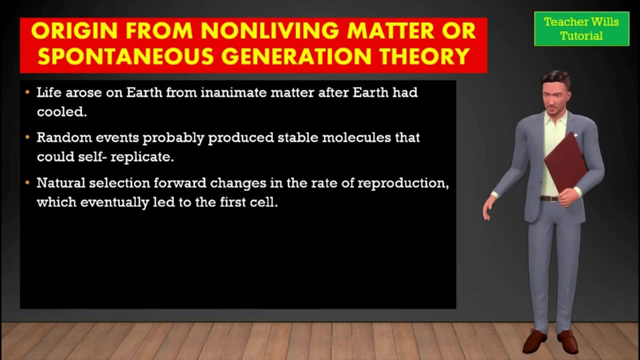 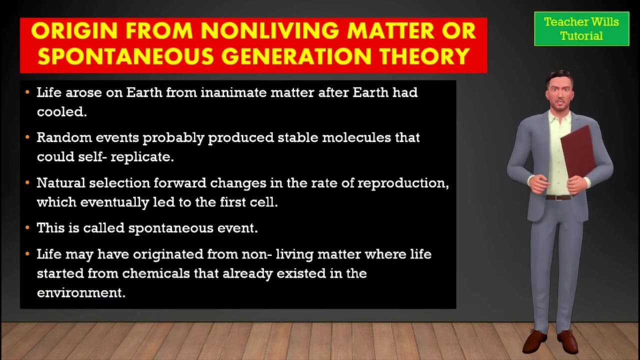 generation theory: Scientists believe that life arose on Earth from inanimate matter. after Earth had cooled, They stated that random events probably produced stable molecules that could self-replicate. Then natural selection forward changes in the rate of reproduction which eventually led to the first cell. This is called spontaneous event, It is believed. 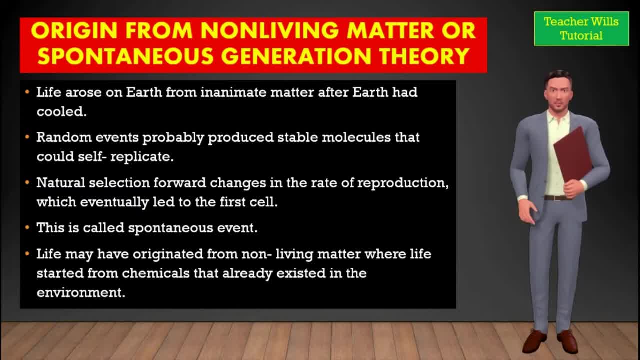 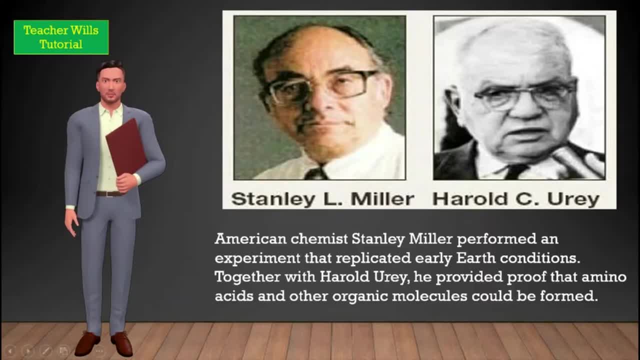 that, under these conditions, life may have originated from nonliving matter, where life started from chemicals that already existed in the environment. American chemist Stanley Miller performed an experiment that replicated early Earth conditions. Together with Harold Urey, he provided proof that amino acids and other 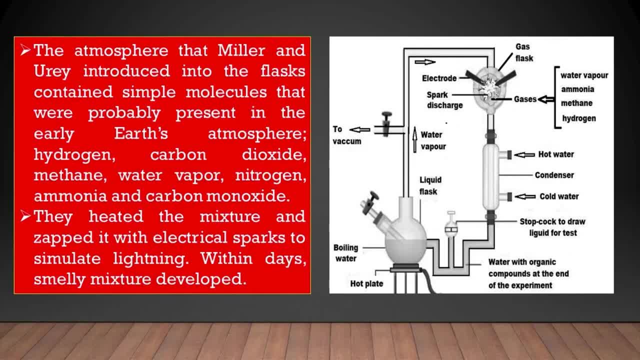 organic molecules could be formed. The atmosphere that Miller and Urey introduced into the flasks contained simple molecules that were probably present in the early Earth's atmosphere: Hydrogen, carbon dioxide, methane, water vapor, nitrogen, oxygen, carbon dioxide, methane, water vapor, nitrogen hydrogen. 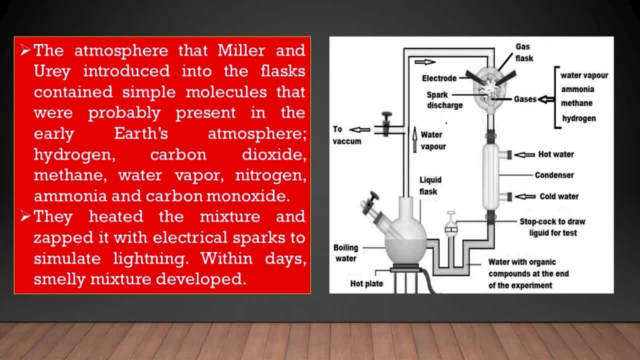 hydrogen carbon dioxide, methane, water vapor, nitrogen, hydrogen, hydrogen, hydrogen, hydrogen hydrogen carbon dioxide, ammonia and carbon monoxide. They heated the mixture and zapped it with electrical sparks to simulate lightning. Within days, smelly mixture developed. 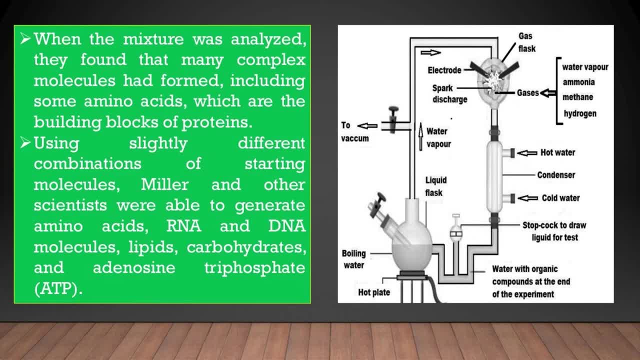 When the mixture was analyzed, they found that many complex molecules had formed, including some amino acids, which are the building blocks of proteins. Using slightly different combinations of starting molecules, Miller and other scientists were able to generate amino acids, RNA and DNA molecules, lipids, carbohydrates and adenosine. 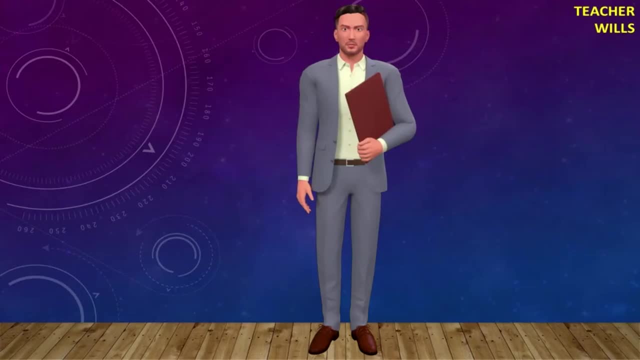 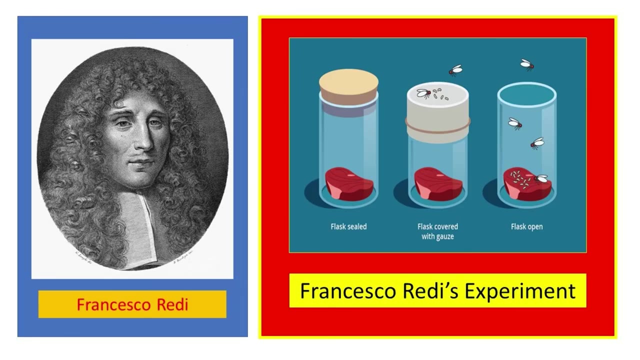 or ATP. There were also experiments made to disprove the spontaneous generation theory, Like, for example, in the year 1968, an Italian physician named Francesco Redi conducted an experiment to see if the theory was true. In his experiment, he put a piece of snake meat, a fish and 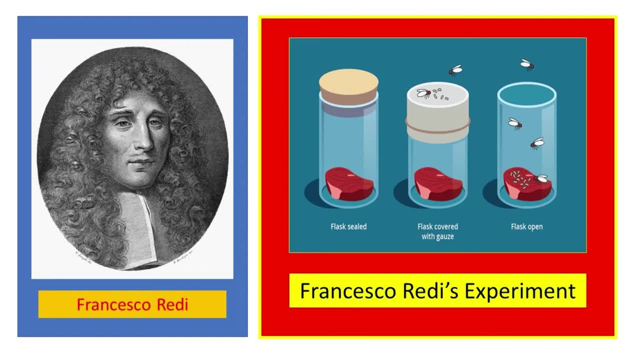 a slice of veal in flasks, covered these with muslin cloth and waited to see if maggots would be developed on the meat. He discovered that maggots grow only if this lay their eggs on it. Lazzaro Spallanzani, Louis Pasteur and John Tyndall performed similar experiments to prove.